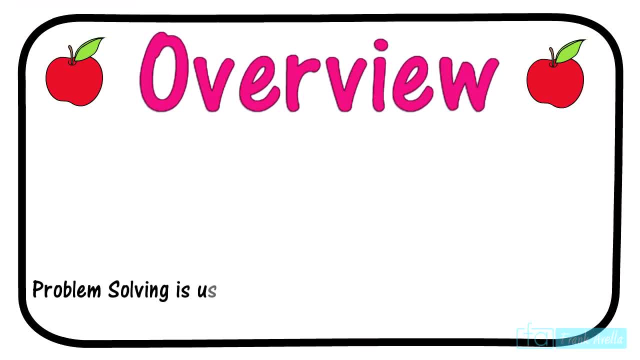 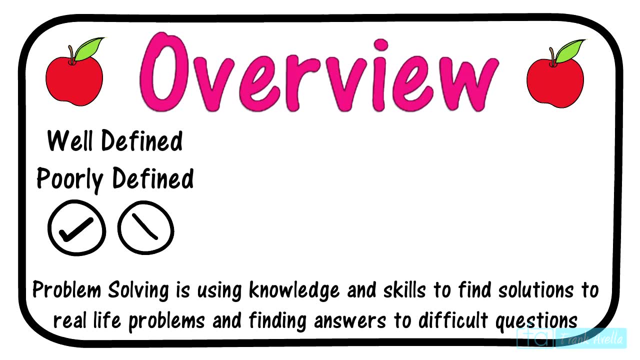 of problem solving. Problem solving is using knowledge and skills to find solutions to real-life problems and finding answers to difficult questions. There are generally two types of classifications: well-defined problems and poorly defined problems. Well-defined ones can be solved. Poorly defined ones may not be solvable In a typical problem to be. 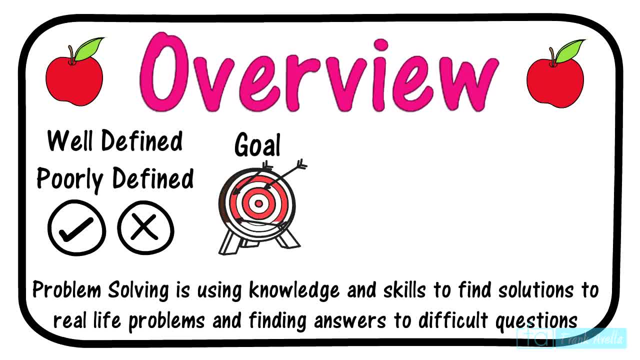 solved, a goal or objective is set for the learner. The objective must be met for successful completion of the problem. Problems require given information. Problems require given information that the learner must make sense of. The learner must also decipher useful and necessary information. 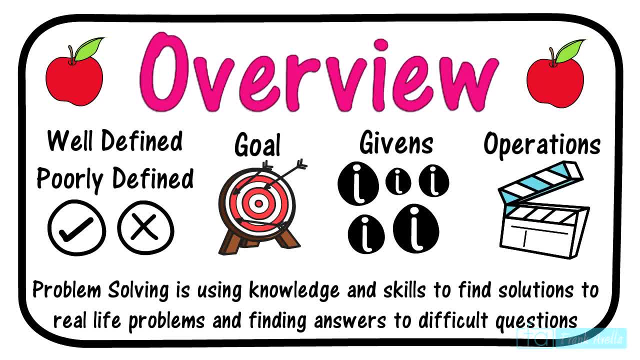 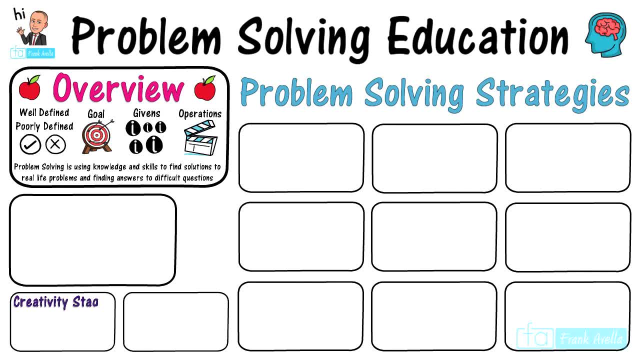 Problem solver is often need various operations in order to arrive at the solution, and these operations don't necessarily have to be mathematical in nature. Next, we'll take a look at some of the creativity stages. The four stages outlined here are credited to Wallace and his work. The first 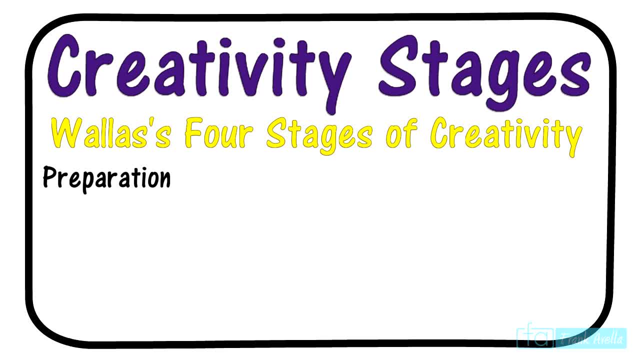 stage is the preparation stage. In this stage, learners look to gather as much relevant information as possible, as well as tapping into whatever prior knowledge they possess. The second stage is incubation, which is basically taking the time to digest information until a moment of insight arrives, The stage after. 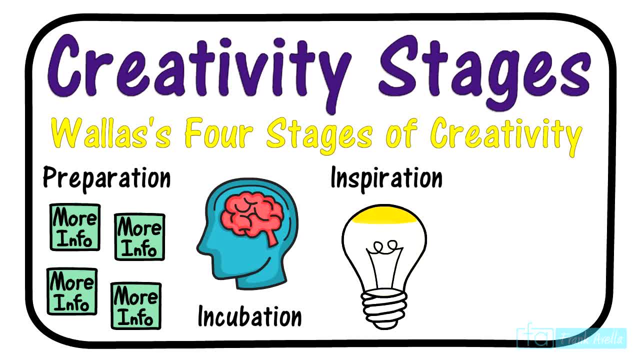 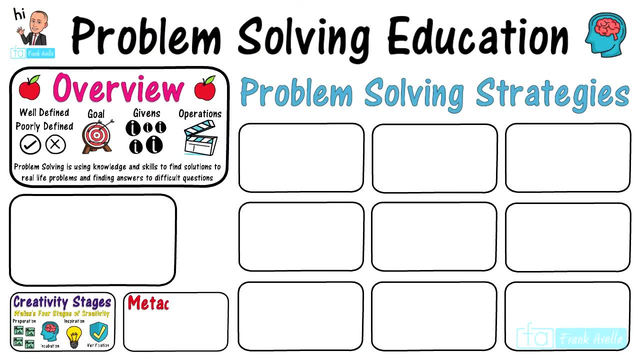 that is, inspiration, or sometimes called illumination. This describes the moment that the learners arrive at a possible solution That leads up to the last stage: verification. Verification of a possible solution that has arisen during the illumination stage. The next section up is metacognition. Generally speaking, metacognition is an awareness or 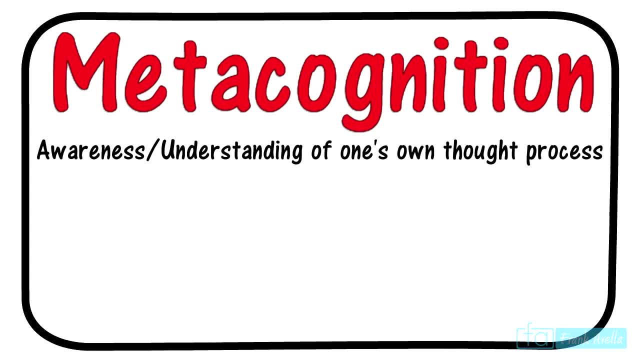 understanding of one's own thought process. Learners that utilize metacognitive strategies develop a confidence to take on challenging problems, and that confidence leads to an increased number of attempts to solving the problem. When you understand your thought process with confidence, you're more equipped to develop plans of action that will take. 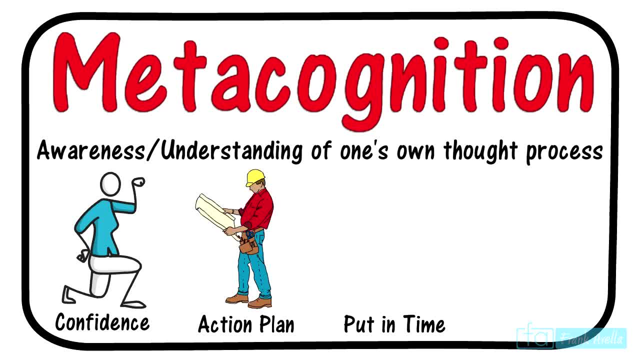 on the problem. Learners using metacognitive strategies are likely to put in more time, and metacognitive learners have that grit to persist until they finish the problem. through Metacognition means being able to monitor one's own self as they go through the problem. 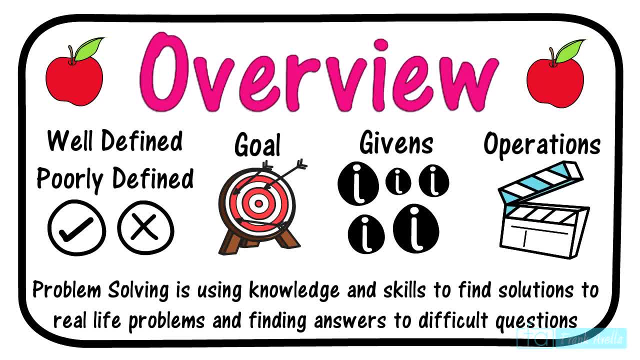 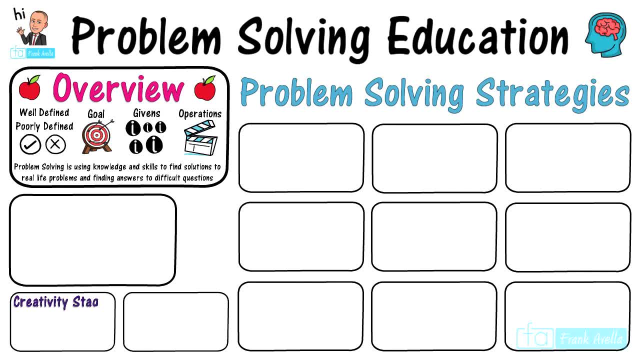 Problem solver is often need various operations in order to arrive at the solution, and these operations don't necessarily have to be mathematical in nature. Next, we'll take a look at some of the creativity stages. The four stages outlined here are credited to Wallace and his work. The first 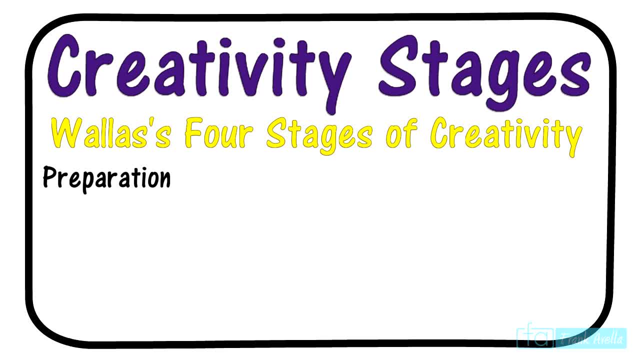 stage is the preparation stage. In this stage, learners look to gather as much relevant information as possible, as well as tapping into whatever prior knowledge they possess. The second stage is incubation, which is basically taking the time to digest information until a moment of insight arrives, The stage after. 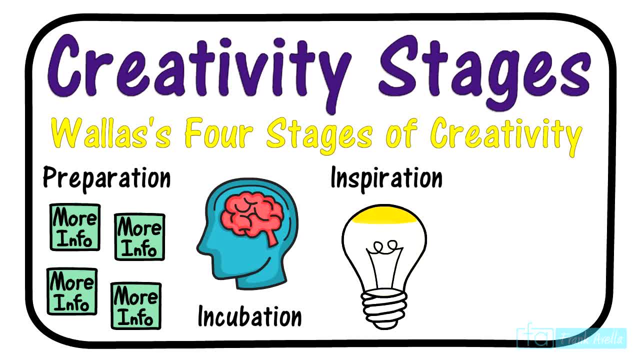 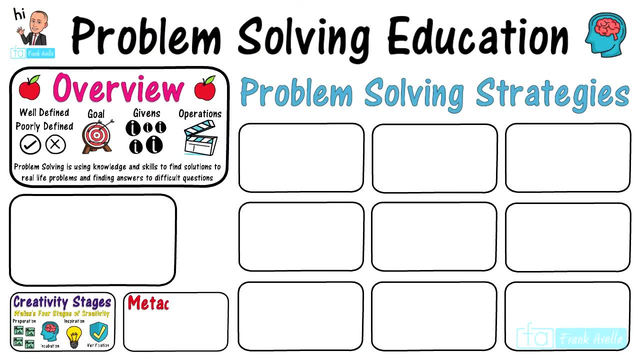 that is, inspiration, or sometimes called illumination. This describes the moment that the learners arrive at a possible solution That leads up to the last stage: verification. Verification of a possible solution that has arisen during the illumination stage. The next section up is metacognition. Generally speaking, metacognition is an awareness or 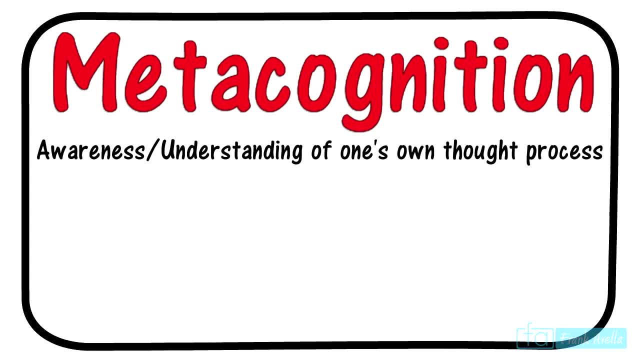 understanding of one's own thought process. Learners that utilize metacognitive strategies develop a confidence to take on challenging problems, and that confidence leads to an increased number of attempts to solving the problem. When you understand your thought process with confidence, you're more equipped to develop plans of action that will take. 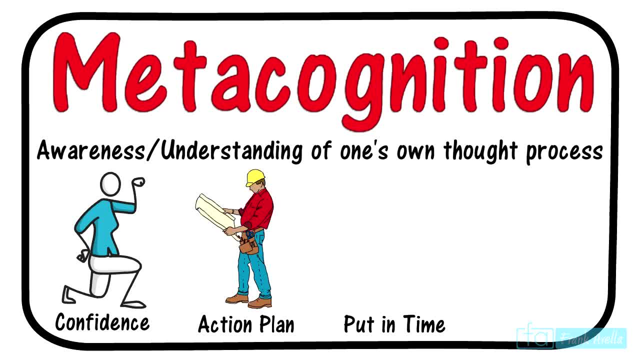 on the problem. Learners using metacognitive strategies are likely to put in more time, and metacognitive learners have that grit to persist until they finish the problem. through Metacognition means being able to monitor one's own self as they go through the problem. 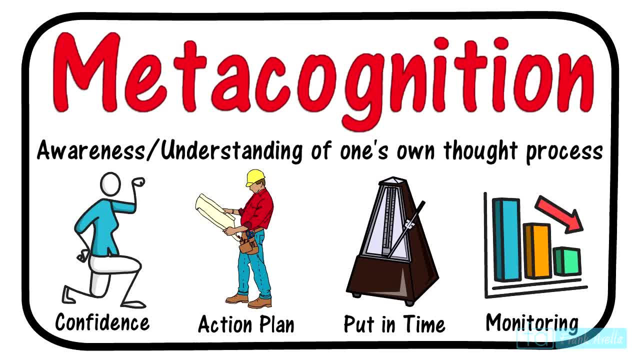 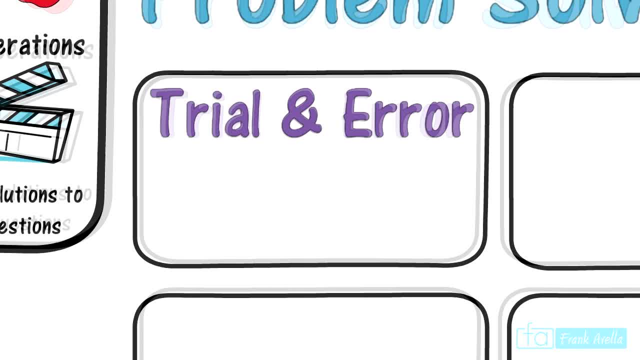 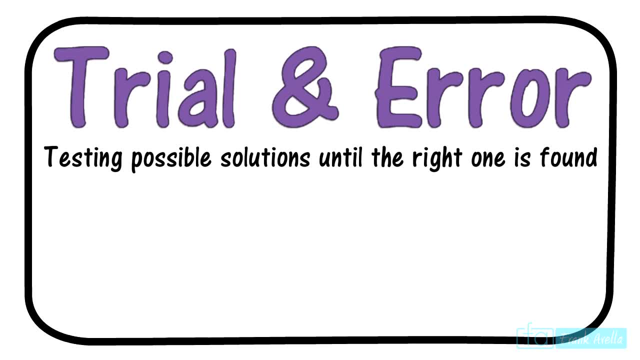 solving process, The learners evaluate themselves as they attempt to solve this issue. Now onto the first of several different problem solving strategies, which is trial and error. Trial and error is essentially testing possible solutions until the right one is found. Thomas Edison is one example of an individual using the trial and error process, as he tried and 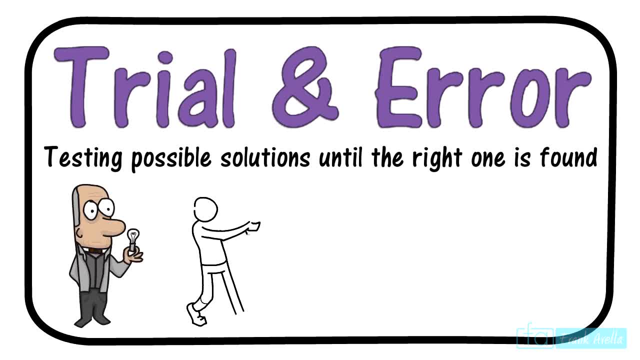 failed, using different experiments until finally having a successful run. Trial and error is about increasing the number of opportunities in order to achieve a viable outcome. This works best, however, with a small sample size, where the learners will have the time to try many different options. Consider putting a jigsaw puzzle together. 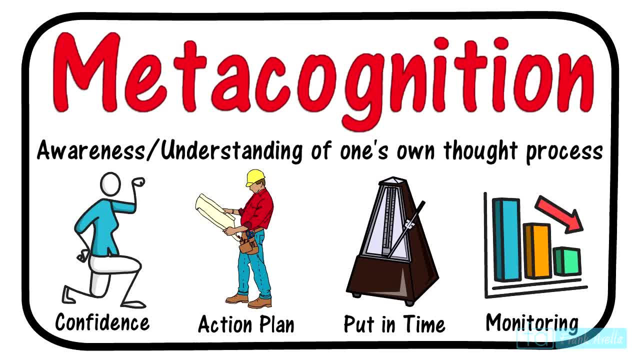 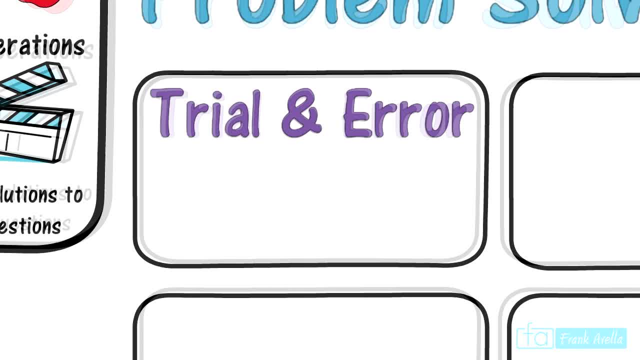 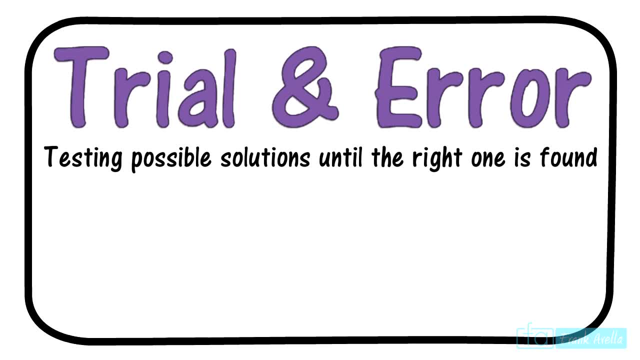 solving process, The learners evaluate themselves as they attempt to solve this issue. Now onto the first of several different problem solving strategies, which is trial and error. Trial and error is essentially testing possible solutions until the right one is found. Thomas Edison is one example of an individual using the trial and error process, as he tried and 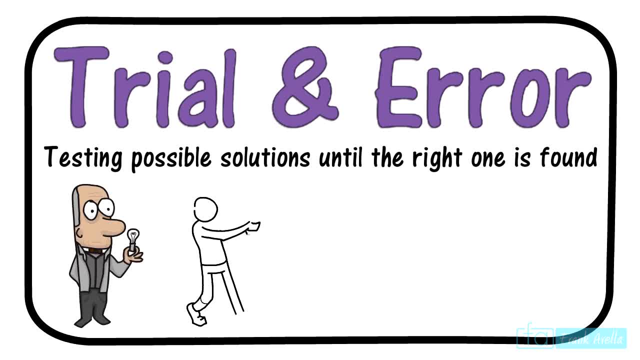 failed, using different experiments until finally having a successful run. Trial and error is about increasing the number of opportunities in order to achieve a viable outcome. This works best, however, with a small sample size, where the learners will have the time to try many different options. Consider putting a jigsaw puzzle together. 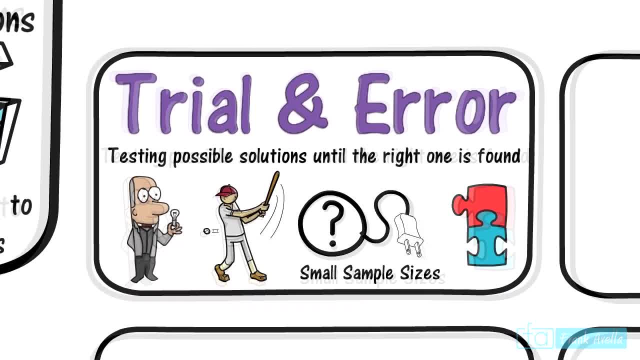 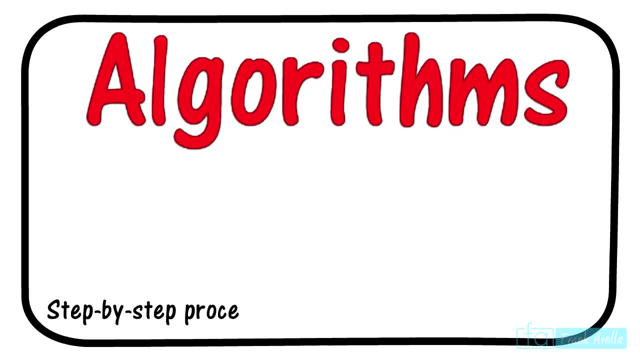 You simply try different pieces until you have the correct one. The next problem solving strategy is using algorithms. Algorithms are a simple step-by-step procedure used for solving specific types of problems. Algorithms are best used for solving well-defined problems. The quadratic formula is actually: 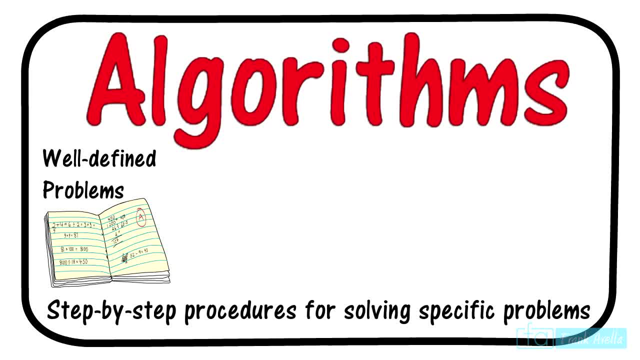 an example of an algorithm because it is a method to solve a problem such as the swing method. Formulas may or may not be considered an algorithm because they specifically involve numbers. Algorithms, on the other hand, don't have to involve numbers. 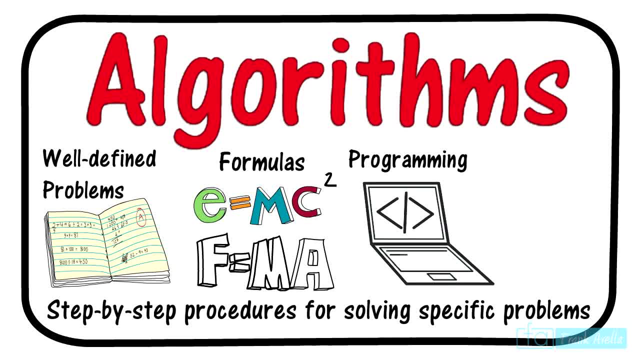 Computer programming is the most common place you'll find the repeated use of algorithms. Various types of engineers use these algorithms in their daily work. It is quite common in the field. It is important to find a number of different algorithms being combined to create a larger. 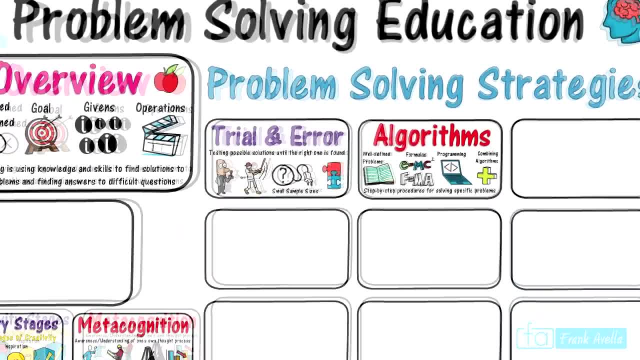 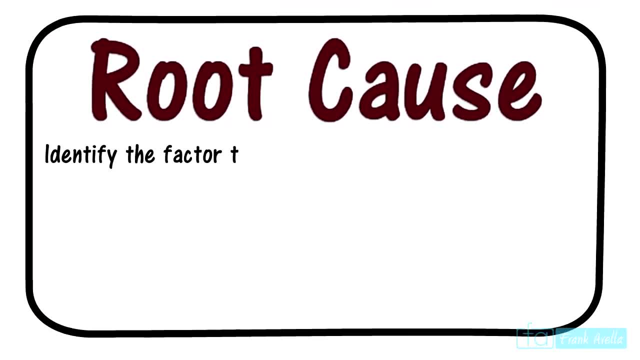 algorithm with a distinct purpose. Continuing on, we come up to the next strategy, which is to identify the root cause. The root cause strategy aims to identify the main factor that is, the cause of the problem. Besides the root cause, there are also additional causes which are not responsible for the 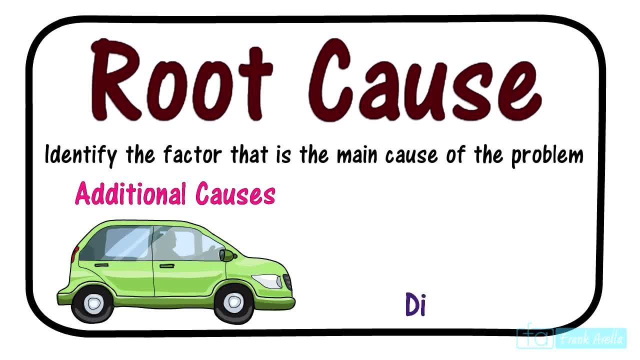 cause of the problem. Learners must differentiate the main cause from additional causes. That is often what you see automatically. Good doctors attack the root cause, not just the symptom. Root cause analysis focuses on identifying the sequence, specifically where the sequence originates, and that goes for. 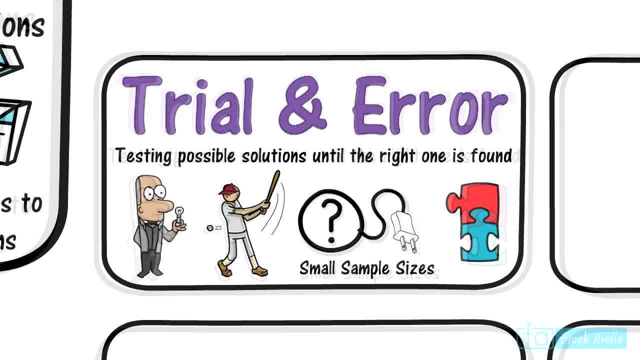 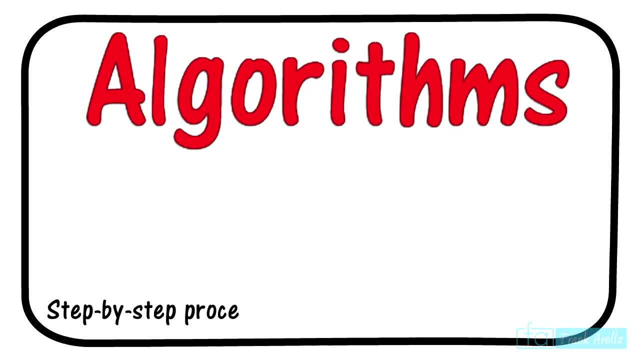 You simply try different pieces until you have the correct one. The next problem solving strategy is using algorithms. Algorithms are a simple step-by-step procedure used for solving specific types of problems. Algorithms are best used for solving well-defined problems. The quadratic formula is actually: 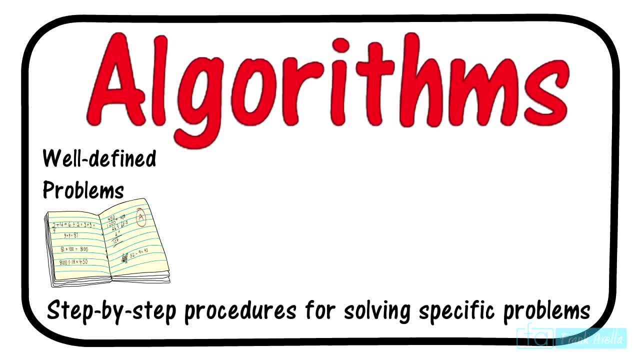 an example of an algorithm because it is a method to solve a problem such as the swing method. Formulas may or may not be considered an algorithm because they specifically involve numbers. Algorithms, on the other hand, don't have to involve numbers. 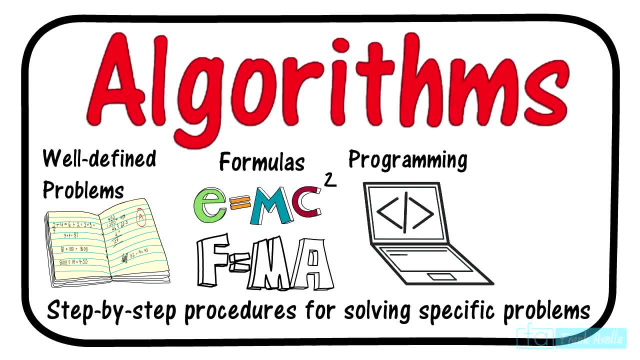 Computer programming is the most common place you'll find the repeated use of algorithms. Various types of engineers use these algorithms in their daily work. It is quite common in the field find a number of different algorithms being combined to create a larger algorithm with a distinct purpose. 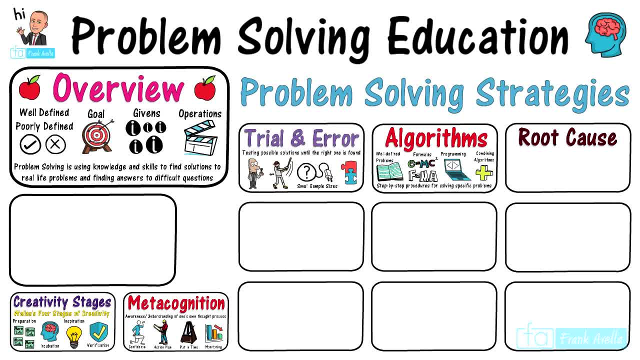 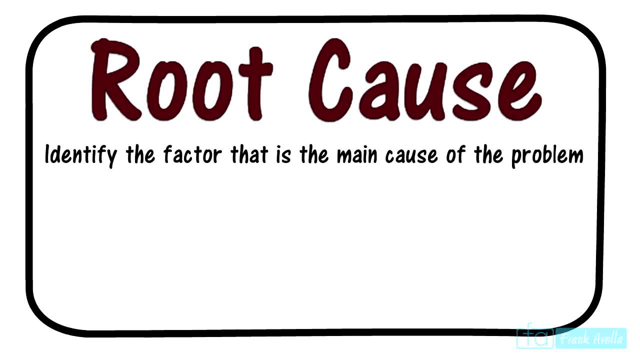 Continuing on, we come up to the next strategy, which is to identify the root cause. The root cause strategy aims to identify the main factor that is the cause of the problem. Besides the root cause, there are also additional causes which are not responsible for the 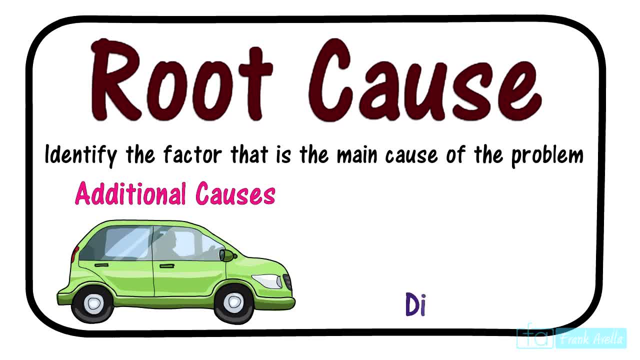 cause of the problem. Learners must differentiate the main cause from additional causes. That is often what you see automobile mechanics doing. Good doctors attack the root cause, not just the symptom. Root cause analysis focuses on identifying the sequence. specifically where the sequence 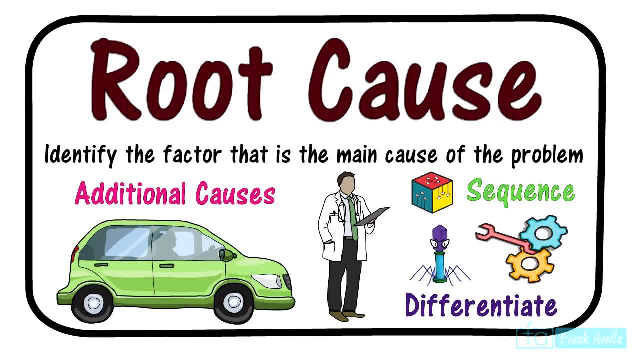 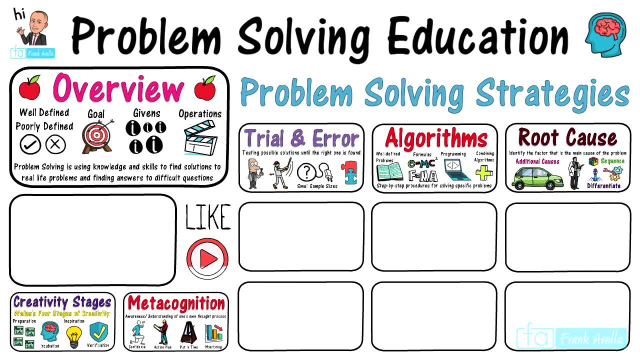 originates, And that goes for the medical field as well. Now, right now, I'm going to take a short break. ask that you hit that like button. don't forget to subscribe to this channel and check the description for links to resources on problem. 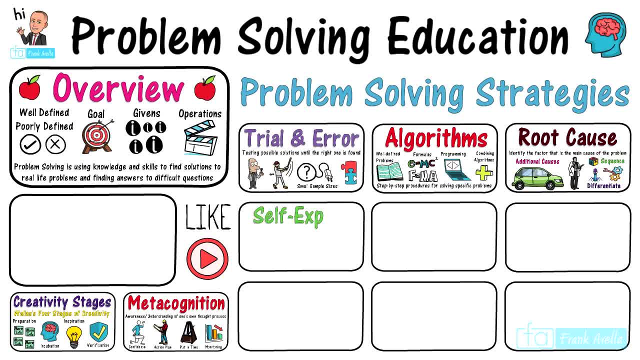 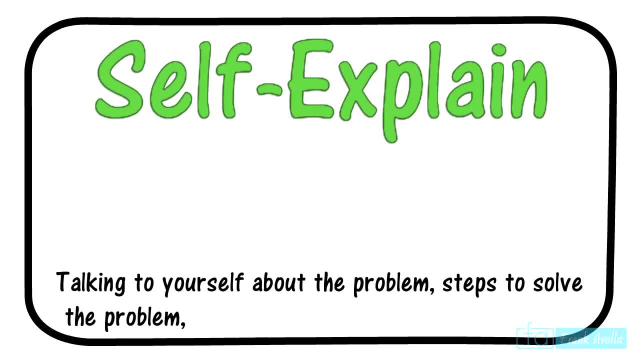 solving. So back to the next problem solving strategy, which is self-talk, Talking to oneself about the problem, steps to solve the problem and what the solved problem will look like. This self-explained strategy is tied to critical thinking. 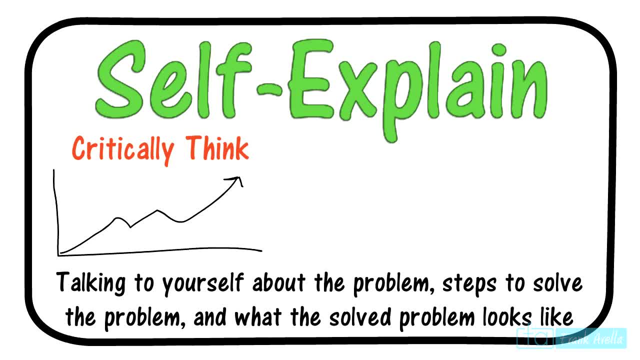 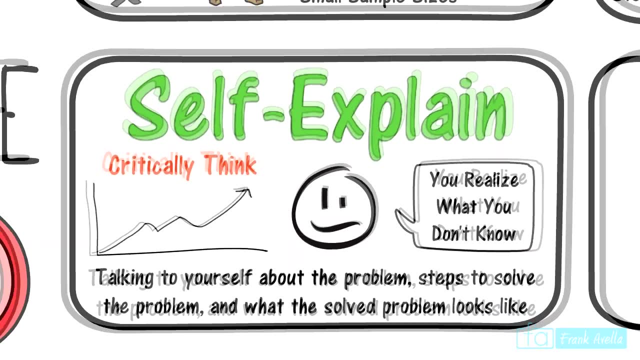 Research has shown that critical thinking is aided by self-talking yourself through a problem. When attempting to solve a difficult problem, it's like you get stuck at one point and it's recommended for learners to use the self-talk strategy at that point. This strategy allows learners to realize that which they do not know. 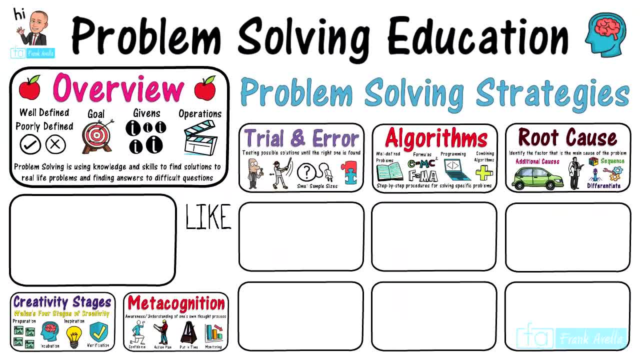 the medical field as well. Now, right now, I'm going to take a short break. ask that you hit that like button. don't forget to subscribe to this channel and check the description for links to resources on problem solving. So back to the next problem-solving strategy, which is self-talk. 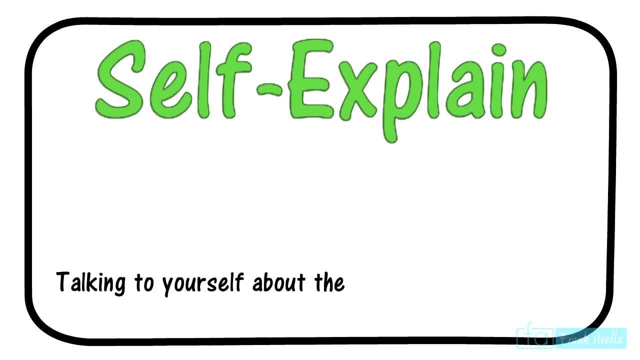 Self-talk, Self-talk, Self-talk, improved self-rawdę, better self-welcoming, like how you solve the problem, steps to solve the problem and what the solved problem will look like. this self explain strategy is tied to critical thinking. 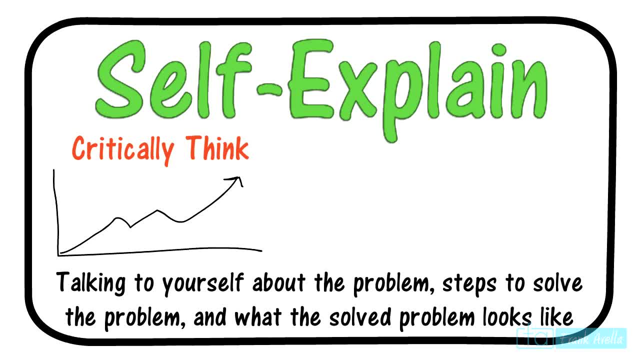 Research has shown to that that critical thinking is aided by self-talking yourself through a problem. When attempting to solve a difficult problem, it's like you get stuck at one point and it's recommended for learners to use the self-talk strategy at that point. 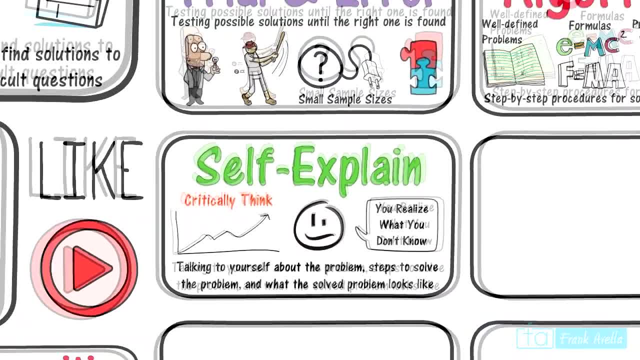 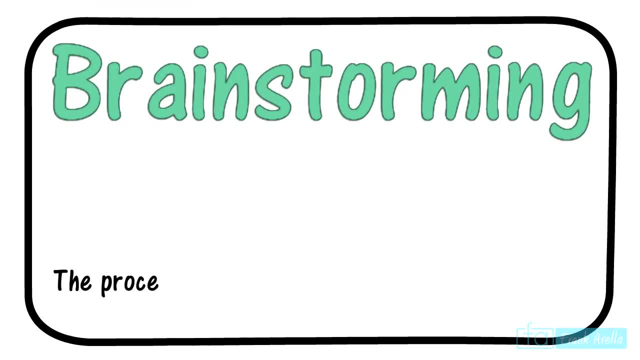 This strategy allows learners to realize that which they do not know. I agree to agree to that because there's something here. Mr N opening sentence. With more strategies coming, the next one up is brainstorming. Brainstorming is the process of collecting a large number of ideas and solutions. 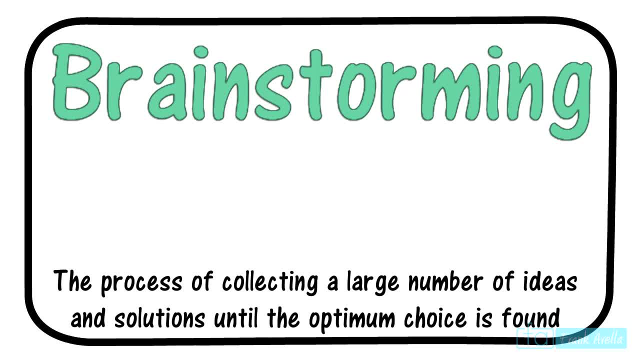 until the optimum choice is found In a whole class brainstorming approach. it's important that there isn't any judgment. You want to get as many ideas out as possible. A person leading a brainstorming session should create a warm and friendly environment. 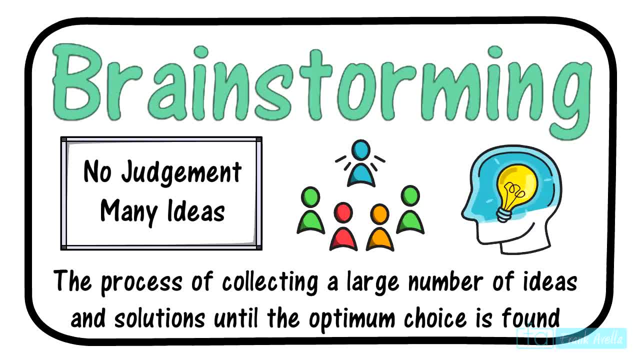 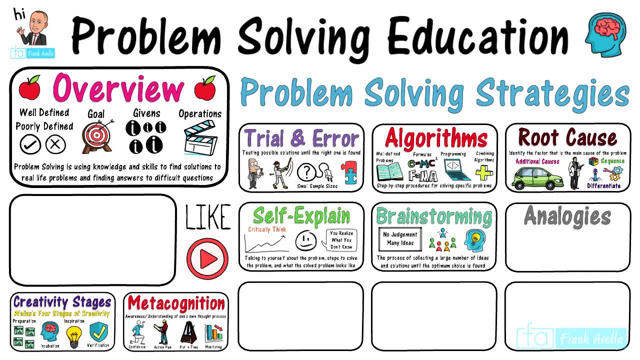 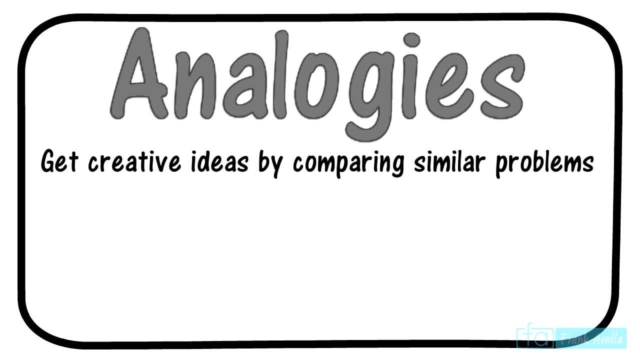 The session should conclude on its own, usually when someone will come up with a mutually agreeable idea. The next problem-solving strategy is to use analogies. Analogies are used to get creative ideas by comparing similar problems. Analogies are described as abstract parallels between two different things, For example: 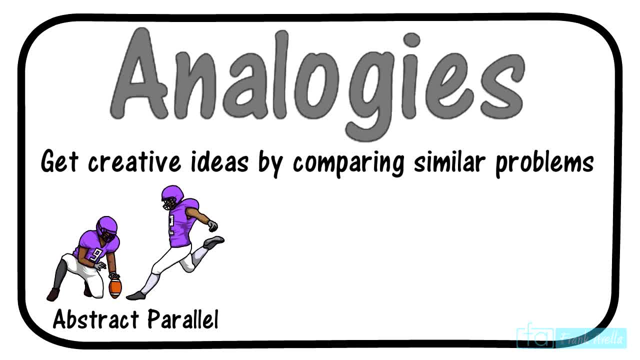 settling for a field goal in football may be similar to settling a case for a lawyer. Using analogies as a problem-solving strategy may occur by the transfer of skills, not just ideas. Also, if a learner used a particular way to solve a similar problem, if they draw an analogy between: 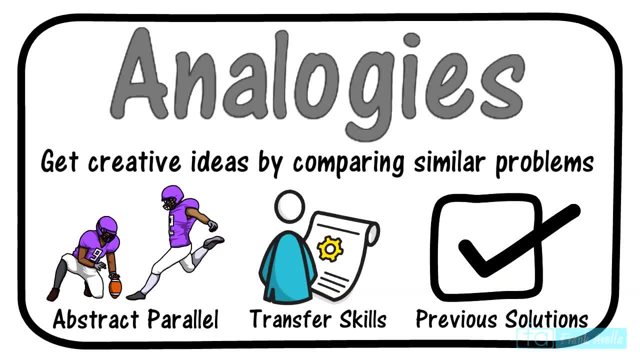 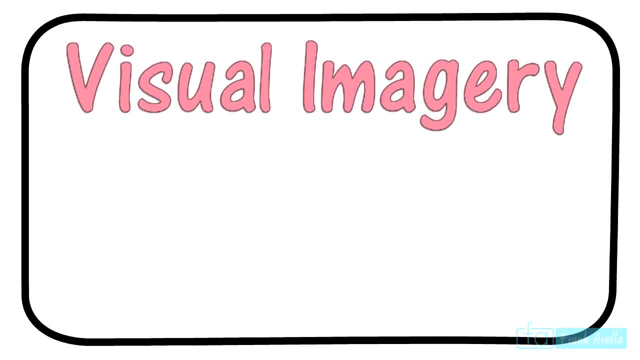 the two, they might be able to use the same method to solve a different or current problem. On to the seventh problem-solving strategy, using visual imagery. Mental visualizations can help facilitate problem-solving. The first benefit of visual imagery is that it will aid. 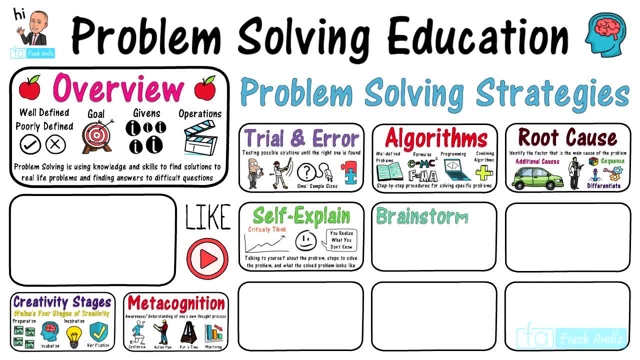 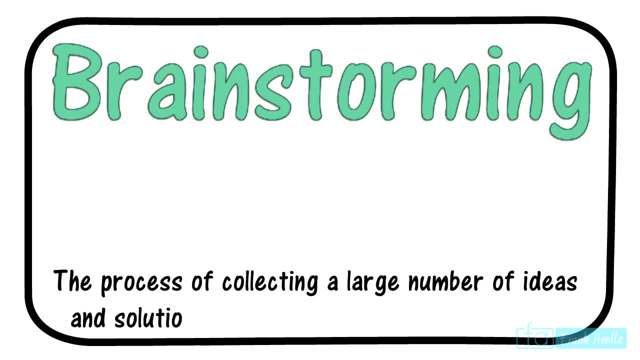 With more strategies coming. the next one up is brainstorming. Brainstorming is the process of collecting a large number of ideas and solutions until the optimum choice is found In a whole class brainstorming approach. it's important that there isn't any judgement. 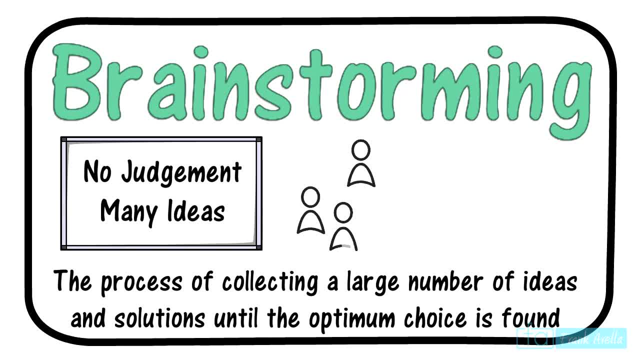 You want to get as many ideas out as possible. A person leading a brainstorming session should create a warm and friendly environment. The session should conclude on its own, Usually when someone will come up with a solution. they will come up with a solution. 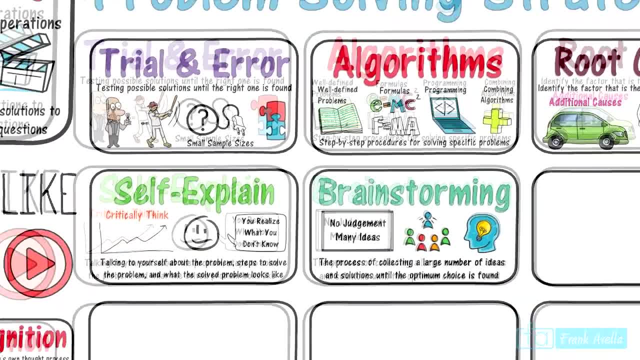 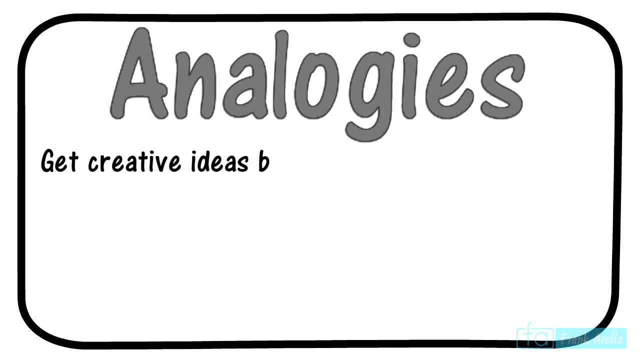 They will come up with a mutually agreeable idea. The next problem-solving strategy is to use analogies. Analogies are used to get creative ideas by comparing similar problems. Analogies are described as abstract parallels between two different things. For example, settling for a field goal in football may be similar to settling a case. 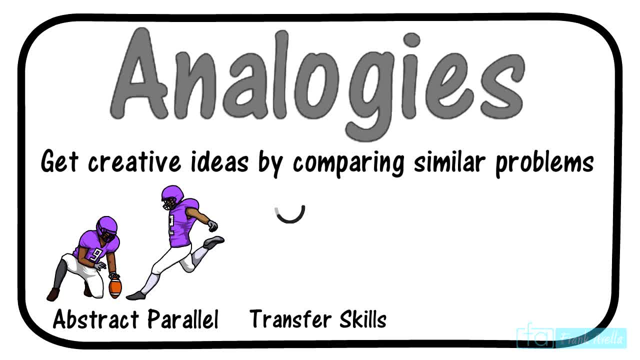 for a lawyer. Using analogies as a problem-solving strategy may occur by the transfer of skills, not just learning. Also, if a learner used a particular way to solve a similar problem, if they draw an analogy between the two, they might be able to use the same method to solve a different or current. 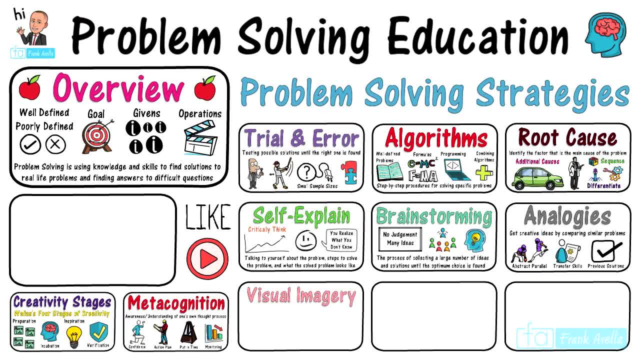 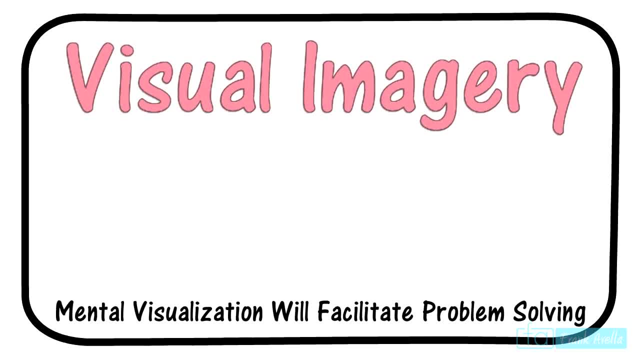 problem. On to the seventh problem-solving strategy: Using visual imagery. Mental visualizations can help facilitate problem-solving. The first benefit of visual imagery is that it will aid in memory retrieval. The visualization may cue the brain to remember relevant and useful information. 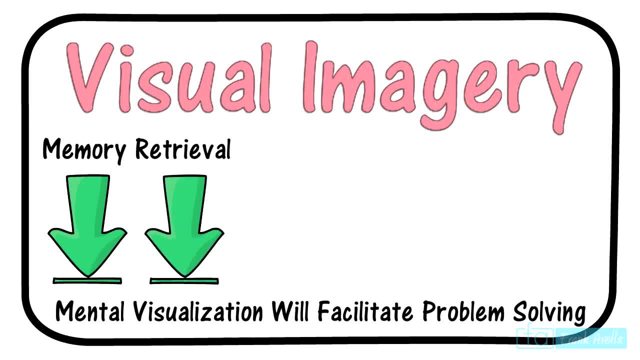 The visualization may cue the brain to remember relevant and useful information. The first benefit of visual imagery is that it will aid in memory retrieval. The visualization may cue the brain to remember relevant and useful information. The visualization may cue the brain to remember relevant and useful information. 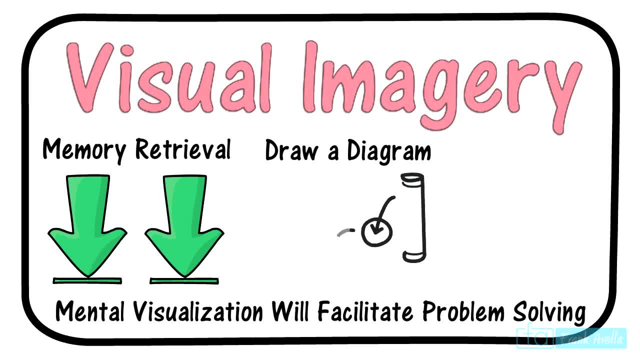 The most common way to use visual imagery is to draw out a diagram. Drawing out a diagram gives the learners a different look at a perspective that can positively impact the way the problem is solved. Drawing a diagram is great for learners with above-average spatial recognition. 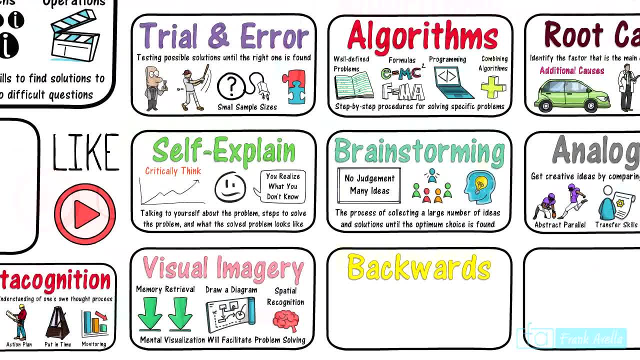 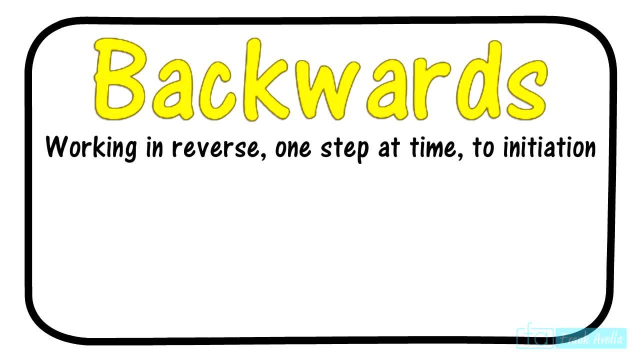 The next problem-solving strategy is to work backwards to solve the problem. Working backwards simply means working in reverse, one step at a time, to the initiation stage of the problem. In mathematics, teachers should encourage students to use this strategy for word problems and other types of problems. 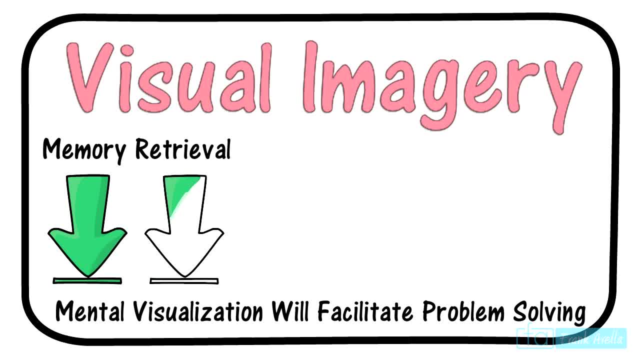 in memory retrieval. The visualization may cue the brain to remember relevant and useful information, as well as the brain to solve the problem. The most common way to use visual imagery is to draw out a diagram. Drawing out a diagram gives the learners a different look at a perspective that 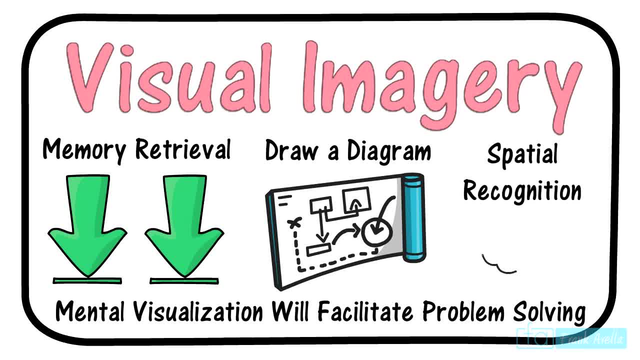 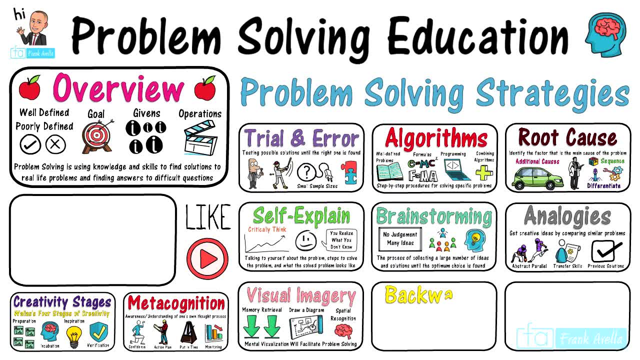 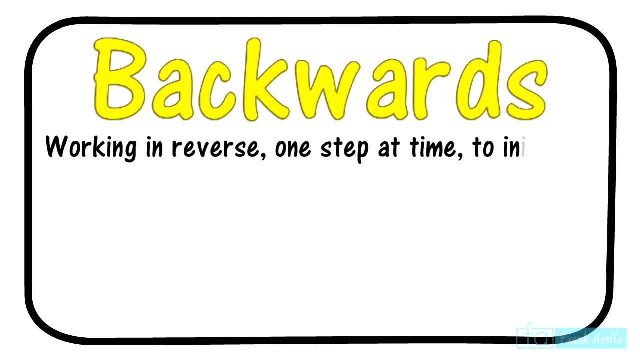 can positively impact the way the problem is solved. Drawing a diagram is great for learners with above-average spatial recognition. The next problem-solving strategy is to work backwards to solve the problem. Working backwards simply means working in reverse, one step at a time, to the initiation stage of the problem. 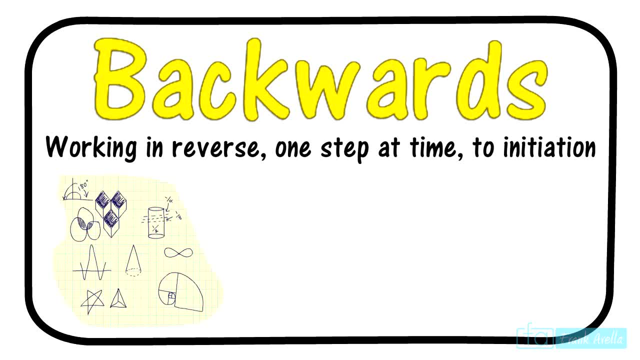 In mathematics. teachers should encourage students to use this strategy for word problems and other types of problems. Another example of a time where working backwards is an optimal method is to finishing a maze. In the business world, backwards thinking is sometimes used as a mean. 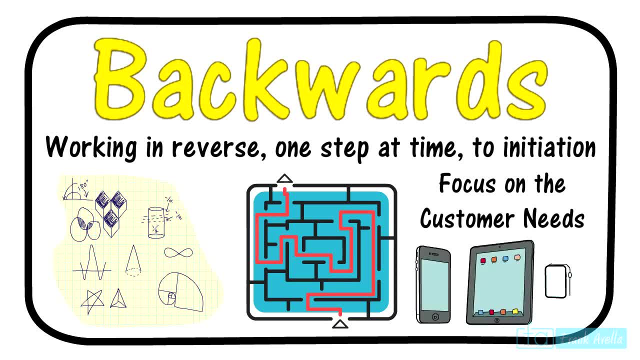 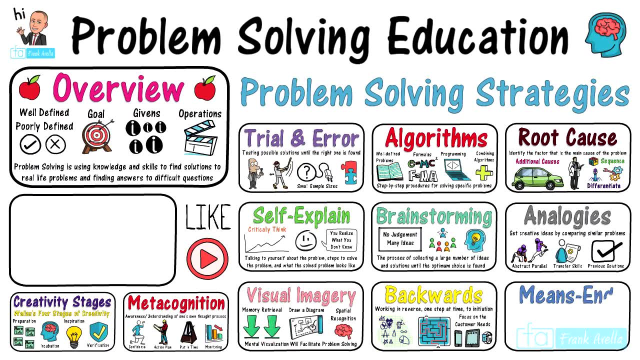 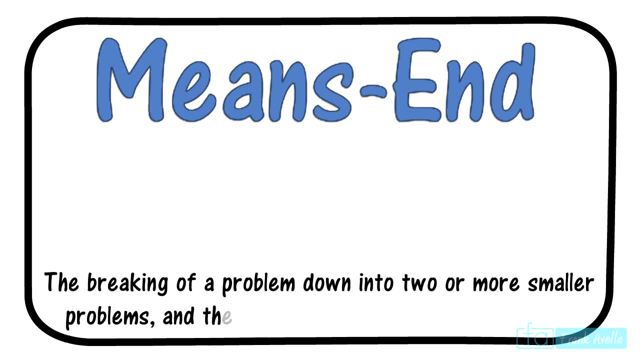 to focus on customer needs. Apple and other technology companies have used this problem-solving strategy in both business and their production model. And now on to the last type of problem-solving strategy mentioned here: means and analysis. It may be described as the breaking of a problem down into two or more smaller problems. 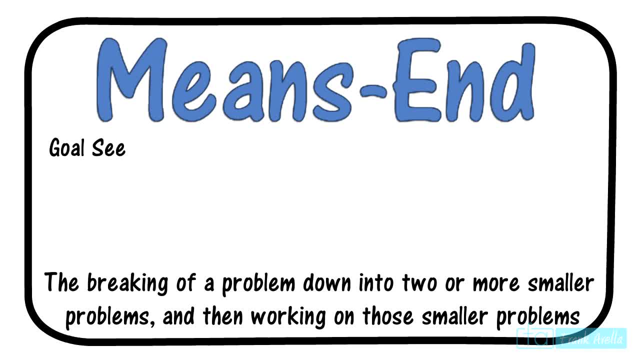 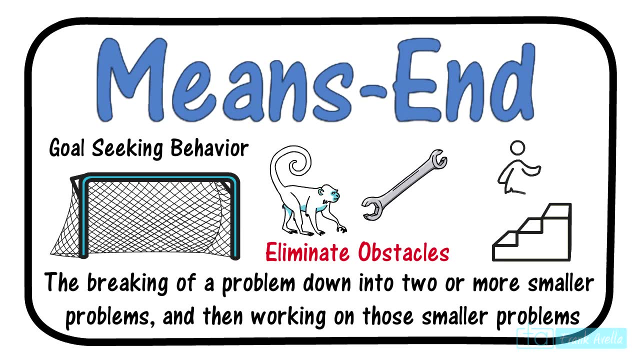 and then working on those smaller problems. Means and analysis focuses on goal-seeking behavior, doing whatever is necessary to get the goal of solving the problem. Obstacles may be eliminated in order to achieve the goal And in this strategy, learners simply solve each problem one obstacle at a time. 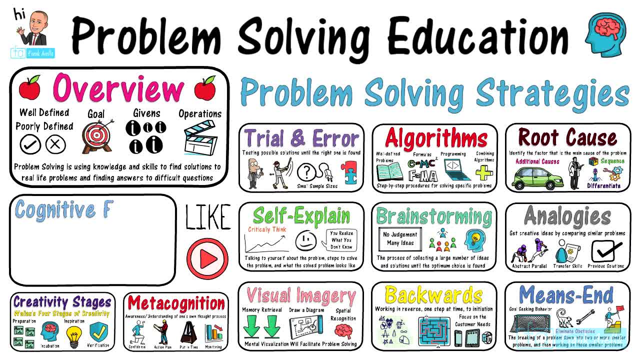 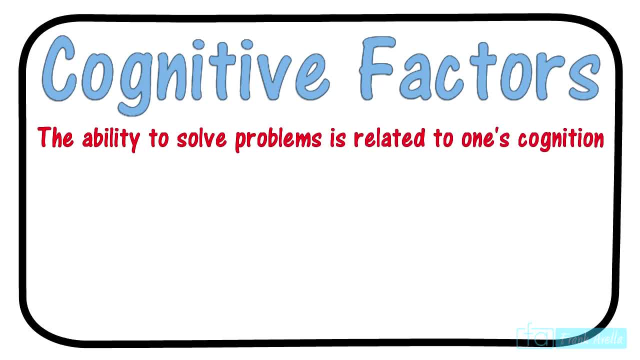 Now, before we finish, let's take a look at some cognitive factors that affect a learner's ability to solve the problem. The ability to solve problems is related to one's cognition. Some factors include confirmation bias, which can prevent learners from solving problems, in that learners don't want to challenge their 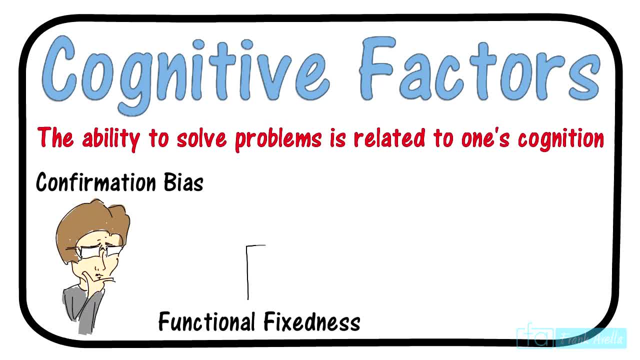 pre-existing views. Functional fixedness is a cognitive bias and it implies that learners will only look at things one way. They won't think outside of the box. The next factor is knowledge based: Having pre-existing knowledge that is related to the problem at hand. 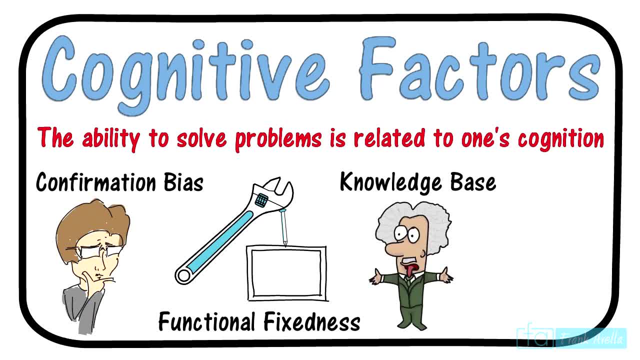 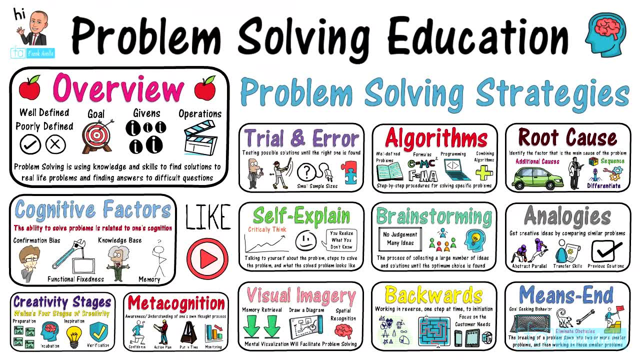 may be necessary to solve the problem. To get prior knowledge, the learner must have a strong memory base, as well as the ability to retrieve that information stored in long-term memory. Anyway, I just want to say again thank you for your time. Don't forget to subscribe to.